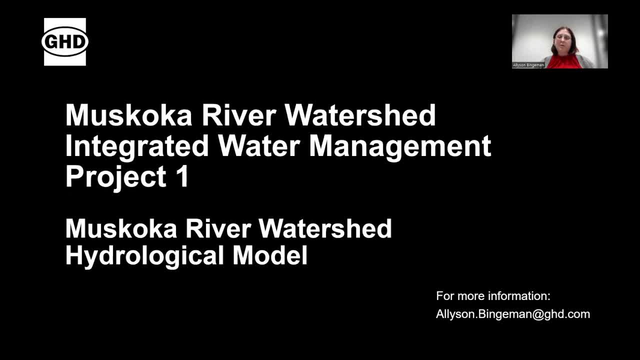 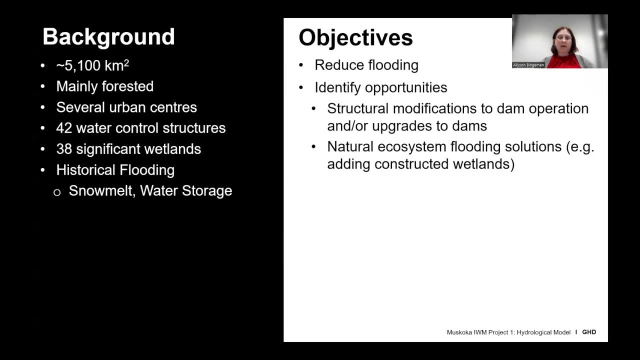 Management Project Number One, which developed the Muskoka River Watershed Hydrological Model. I have also included my email address on this slide. This slide includes two titles and two bulleted lists showing the project background and objectives. The Muskoka River Watershed is just over 5,000 square kilometers in size. 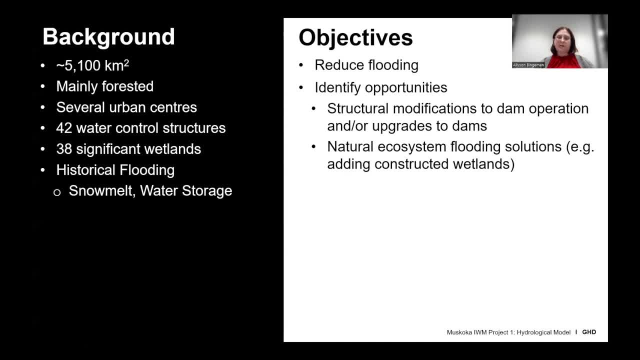 It is mainly forested but has several urban centers. The largest urban centers are Huntsville, Bracebridge and Gravenhurst. The watershed has 42 water control structures and 38 significant wetlands. The watershed has a history of flooding. 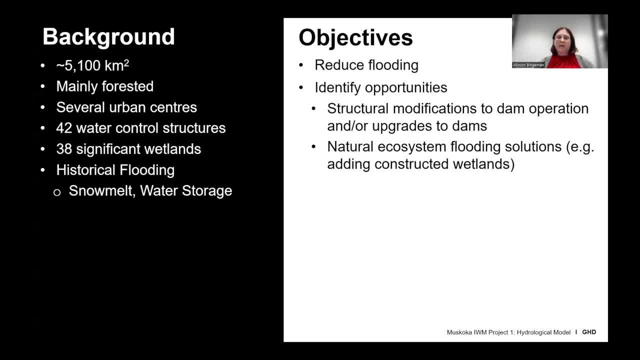 which generally occurred during the spring freshet when there has been insufficient storage. The objective of this project was to reduce flooding, in particular to identify opportunities for flood reduction. The first opportunity was for structural modifications to the dams, either in their operation or changes to the dams themselves. The second opportunity was 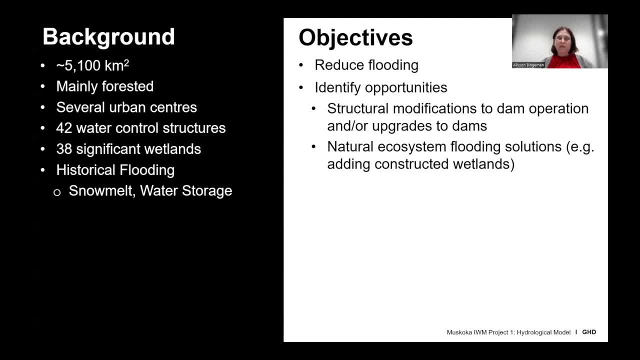 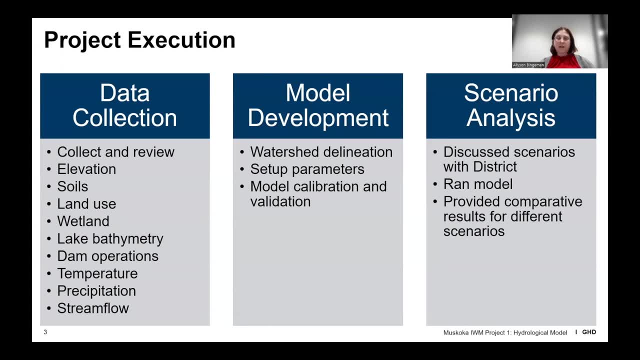 to develop the project's residential and natural ecosystem, flooding solutions such as constructed wetlands. This slide includes a title and a figure describing the stages of project execution. The first stage was data collection. During this stage, GHD collected and reviewed a number of 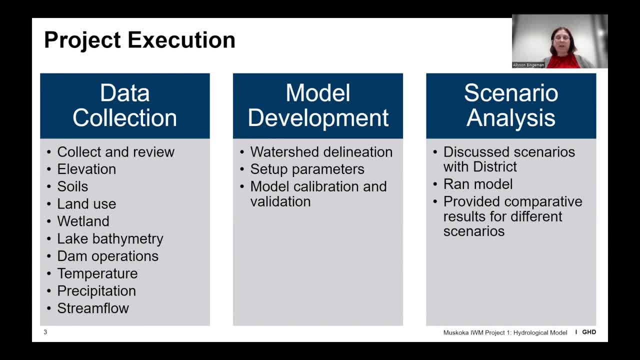 different data sources, including elevation, soils, land use, wetlands, lake bathymetry, dam operations, temperature, precipitation and stream flow. The second stage of project execution was model development, watershed delineation and connecting the watershed within the software, then selecting equations for the different hydrological processes and setting up their parameters, and then, finally, model calibration and validation. 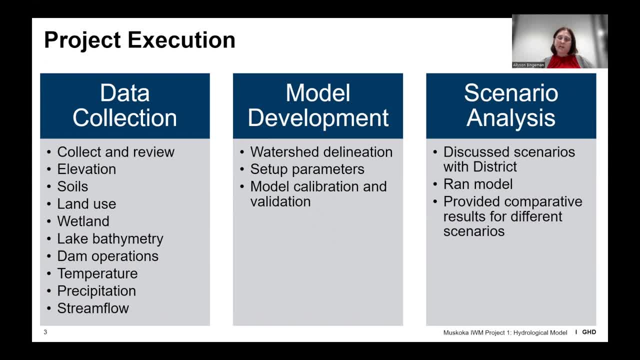 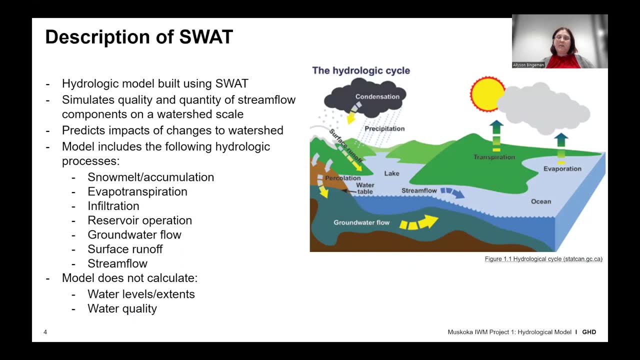 The third stage of project execution was scenario analysis. GHC discussed a number of scenarios for the district and selected the ones to include in the project, ran the scenarios and then provided comparative results. This slide includes a title, a bulleted list and a figure showing the hydrological cycle. 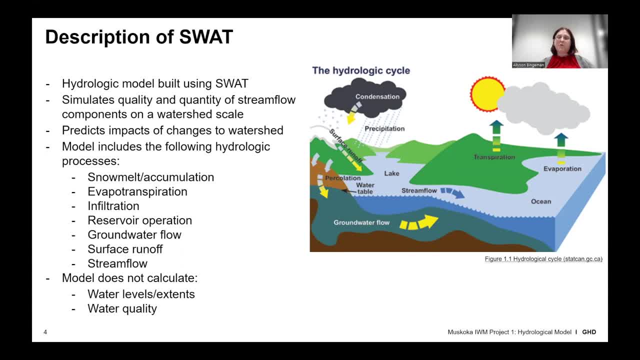 The model was built in SWAT, which stands for Soil Water Assessment Tool. SWAT can simulate water quality and water quantity for various streamflow components on a watershed scale. It can also predict the impact of changes to the watershed on streamflow. The model includes the following hydrological processes: 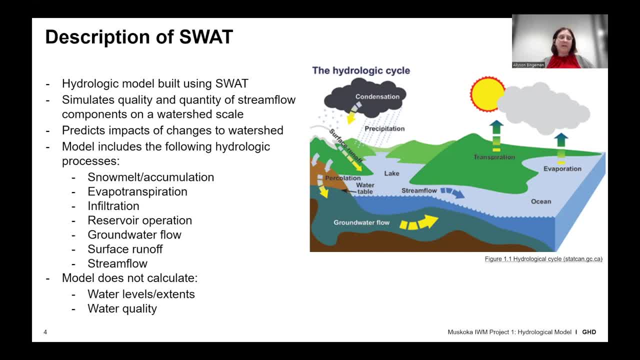 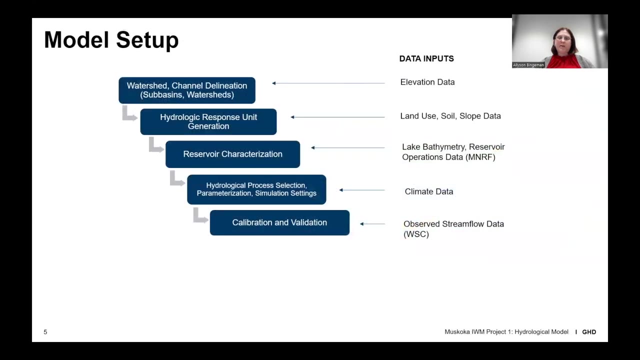 Snowmelt and accumulation, Evapotranspiration, Infiltration, Reservoir operation, Groundwater flow, Surface runoff And streamflow. The model does not calculate water levels or flooding extents And, although SWAT can calculate water quality, the model has not been set up for water quality calculation at this time. 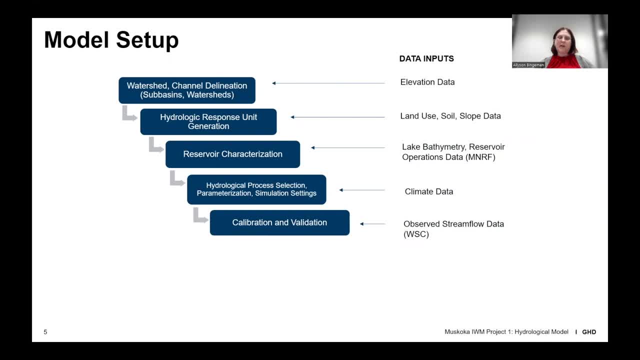 This slide includes a title and a figure describing the stages of model setup. The first stage of model setup is the delineation of watersheds. This is a model using both the streamflow and the water supply and the zones in the water and channels. 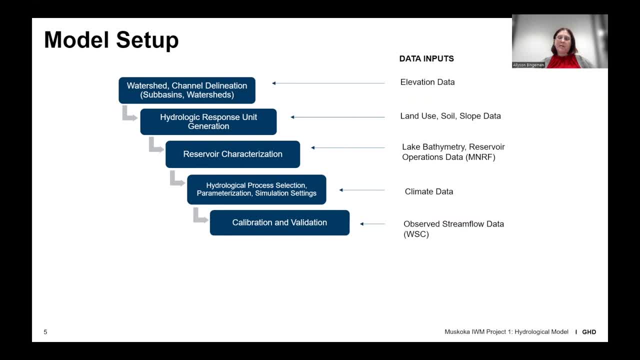 And connecting them together in the software. This stage used the elevation data as input. The second stage is the generation of hydrological response units. A hydrological response unit is an area within a watershed with similar land use, soils and slopes. The area does not have to be contiguous. 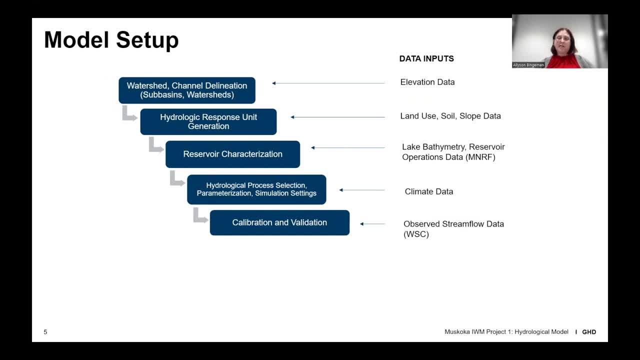 third stage is reservoir characterization. For this stage, we imported the lake bathymetry and set up the reservoir operation. The fourth stage includes selecting the equations for the various hydrological processes, setting up the initial parameters and setting up the simulation itself. 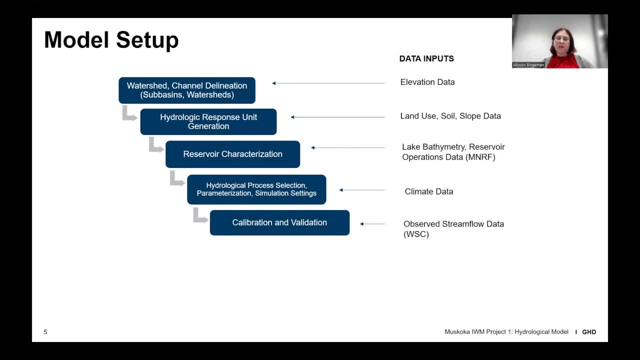 For this stage, the climate data were imported into the model. The final stage of model setup was model calibration and validation. This stage involved modifying the parameters so that the streamflow is matched to the observed streamflow. This slide includes a title and a bulleted list. 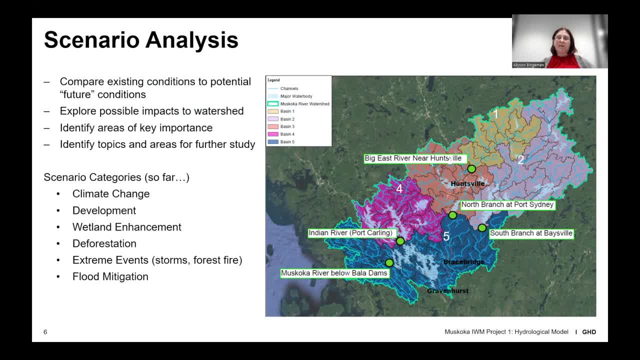 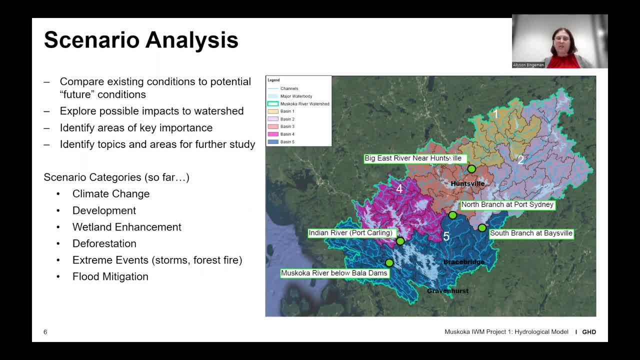 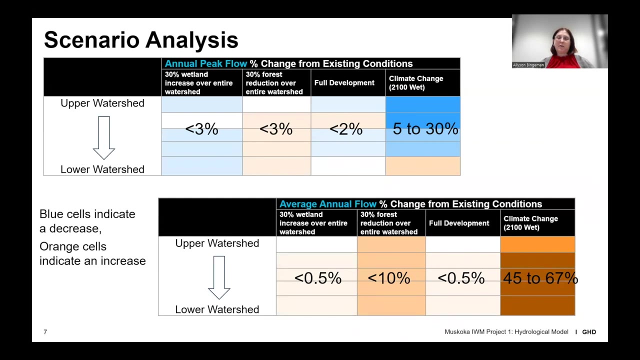 can be identified, along with other topics or areas that should be studied further. For this project, several categories of scenarios were studied, which included climate change, development of each of the urban areas, wetland enhancement, deforestation, extreme events such as storms and forest fires, and flood mitigation. This slide includes a title and two figures showing the relative. 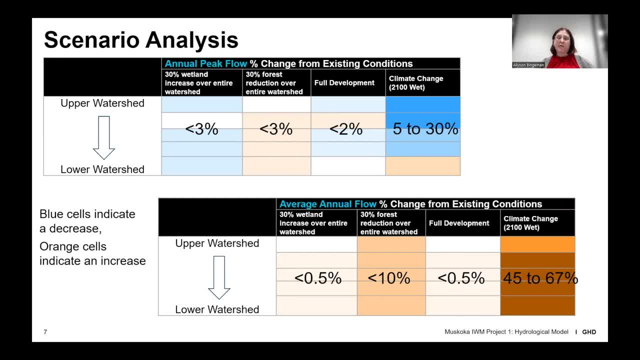 changes in peak flow or average flow for different scenario categories. The scenario analysis indicates that there would be relatively small changes in peak flow and annual flow due to wetland increase, deforestation or developing each of the urban areas to their full extents. Even relatively large changes in wetlands and forests produce relatively small changes in peak flow- up to a 3% change- and average flow up to a 10% change. 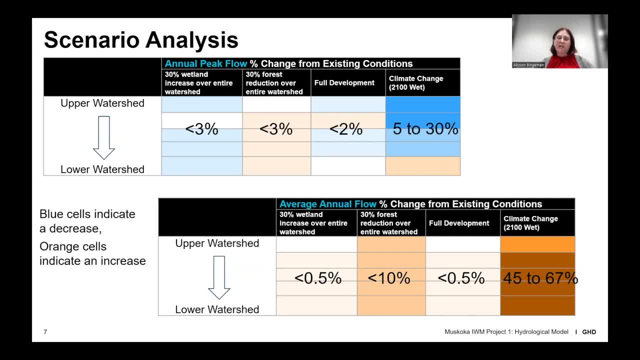 In comparison, the projected changes for the climate change scenarios are much larger. For peak flow, the changes are between a 5% and 30% reduction in peak flow and 45% to 67% increase for annual flow. Since climate change was the largest factor analyzed in the scenario analysis, we will describe it further. 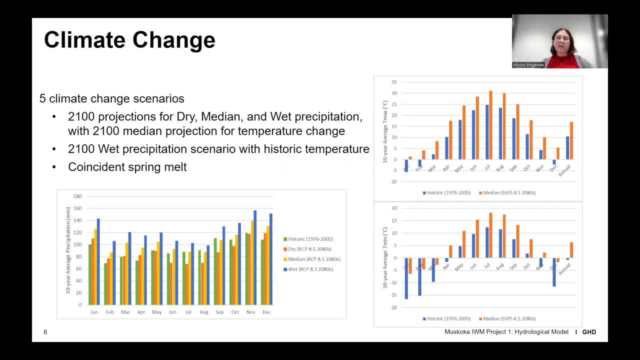 This slide contains a title, a bulleted list describing the climate change scenarios and three figures showing the changes in precipitation and temperature. The scenario analysis includes five scenarios. The first three scenarios incorporated three different projections taken from global climate model data for precipitation: dry, median and wet, combined with the median projection for temperature. 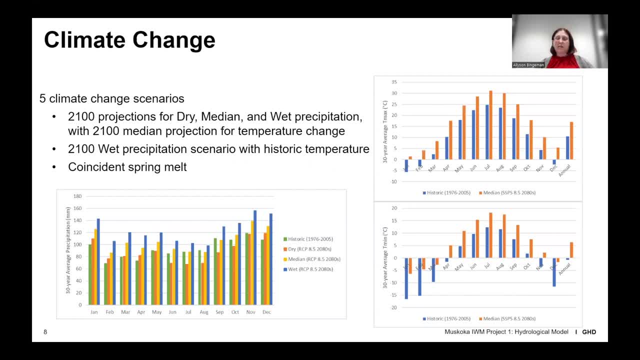 The fourth scenario used the wet projection for precipitation with historic temperature. The final scenario included a coincident spring melt. Historically, spring melt has proceeded from south to north across the watershed. This scenario explores the impact of spring melt occurring at the same time throughout the watershed. 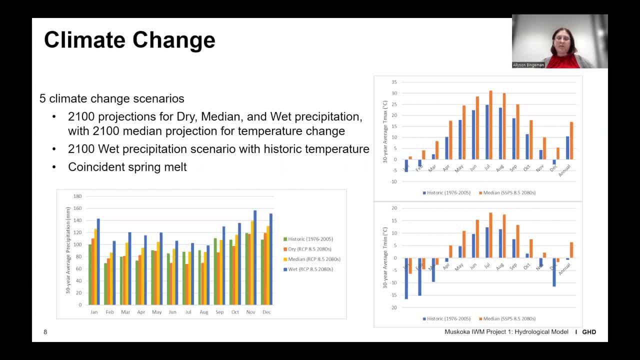 The first figure shows the precipitation for each month of the year for historic dry projection, median projection and wet projection. The dry projection is generally lower than the historical precipitation, with small increases in the winter months. The median projection is higher than historical precipitation for most months of the year. 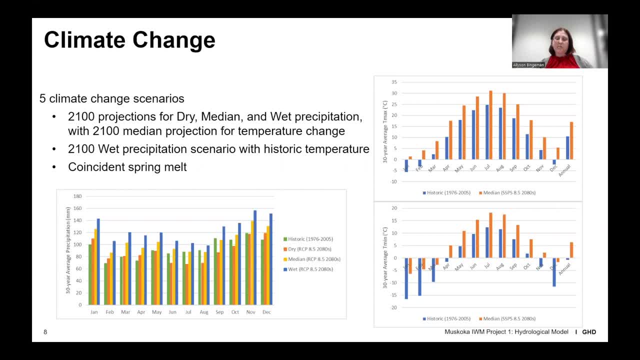 The wet projection has a large increase in precipitation throughout the year. The second and third figures show the increase in temperature for each month of the year. Throughout the year, the global climate model data projects an increase in temperature of six to seven degrees Celsius. 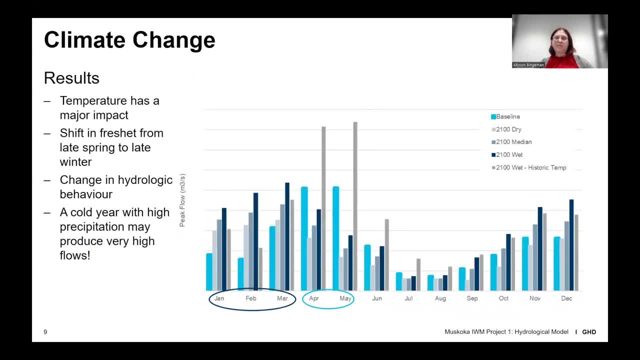 This slide includes a title and a bulleted list. It also includes a figure showing the peak flow in each month of the year for various climate change scenarios. The results show that the projected changes in temperature have a major impact on streamflow. Historically, the spring freshet has occurred in April or May. 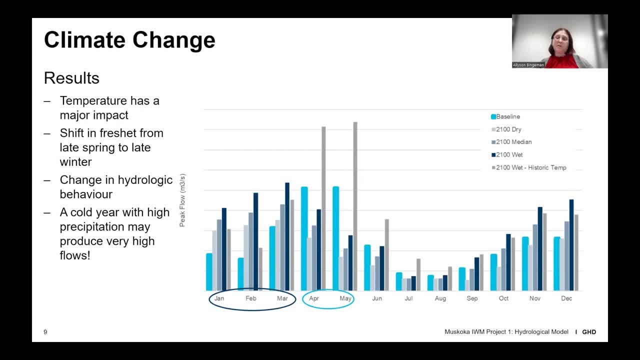 And resulted in the highest annual flows in the watershed. Under climate change, the spring freshet has moved to earlier in the year. January to March. The snow accumulation is much lower and the snow melts more frequently. Some winter precipitation also falls as rain. 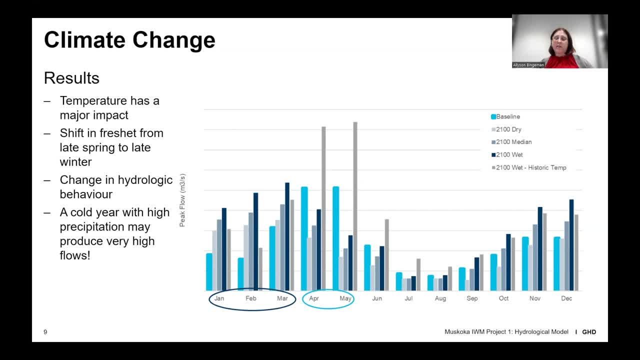 This results in a change in the hydrological behavior, with increased winter streamflow and decreased spring and summer streamflow. In the scenario that used historical temperature, which would represent an extremely cold year, we see that the increased winter precipitation results in a large snowpack and a very large spring freshet. 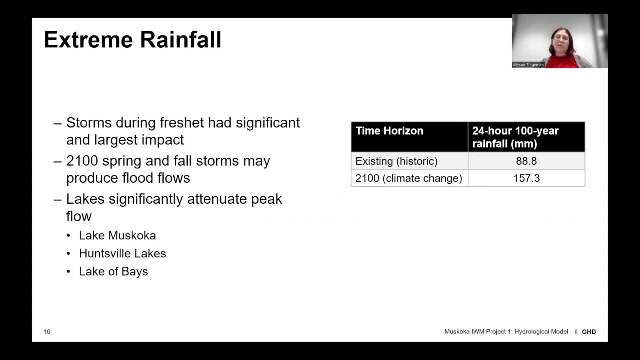 This slide contains a title and a bulleted list. It also shows a table comparing the extreme rainfall events for both the historic period and the future climate change period. Historically, the 24-hour 100-year rainfall event was approximately 89 millimeters. 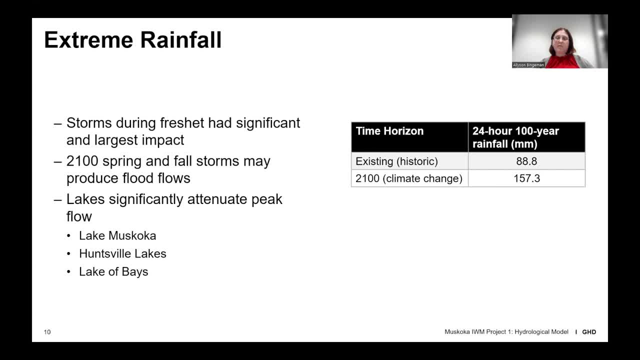 Under climate change. it is expected that the 24-hour 100-year event could increase to 150 millimeters In the extreme rainfall scenarios. the climate change 24-hour 100-year event was placed in the model at various locations and at various times in the year. 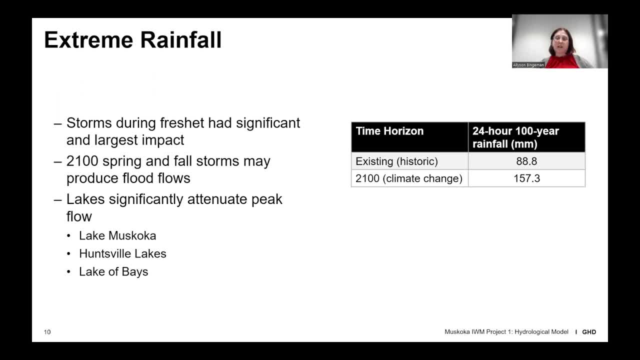 Historically, extreme events occurring during the spring freshet have resulted in the highest flow rates Under climate change. this will still occur, although the spring freshet has moved earlier in the year, so the storm would also need to occur earlier in the year. 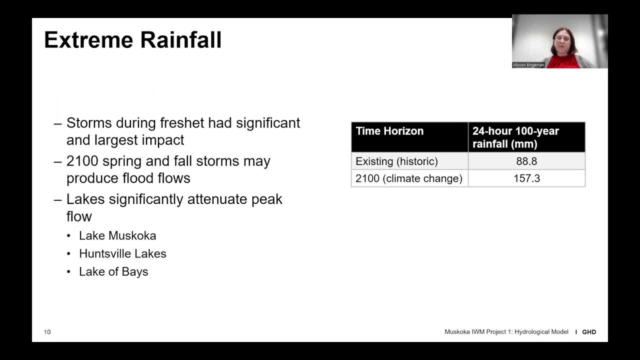 However, the results indicate that the spring freshet has moved to the north of the year. The late summer and fall events can also produce high flow rates. These results are particularly key because the large lakes in the watershed have historically been used to attenuate peak flows. 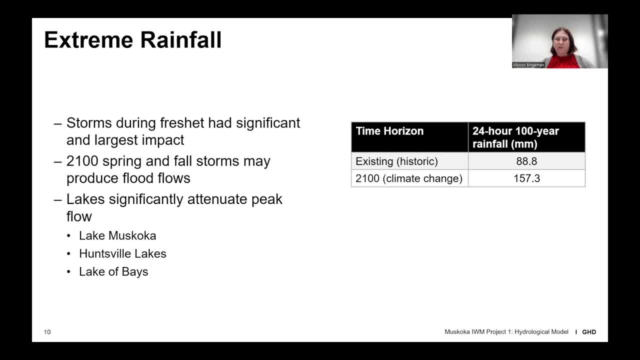 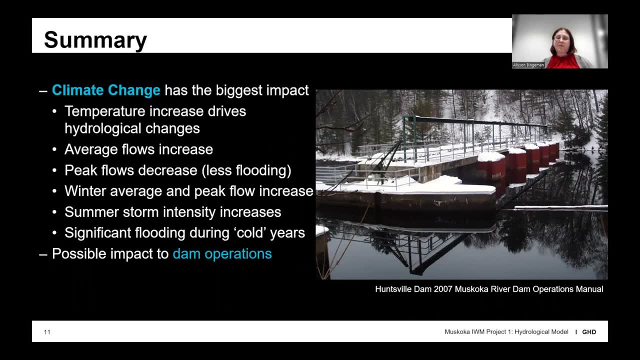 However, they are generally close to full during the summer and fall. This slide contains a title and a bulleted list summarizing the scenario analysis. It also contains a photo of the Huntsville Dam. It was found that climate change has the largest impact on stream flow as compared to the other scenarios tested.